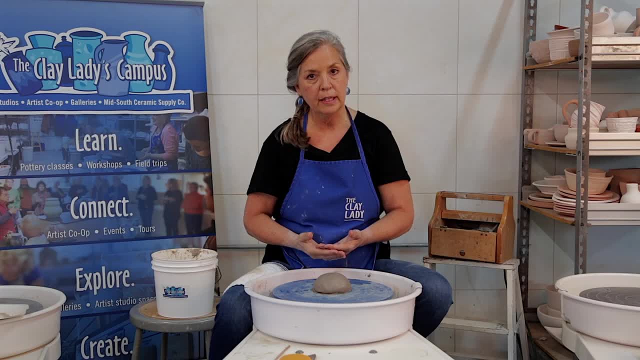 the play they can cheer, lead After the potter gets finished making their pot. then the coach becomes the potter. They switch and they switch until the end of our time. I also teach the kids on the potter's wheel, the Clay Lady way, where the kids will make their pot on the 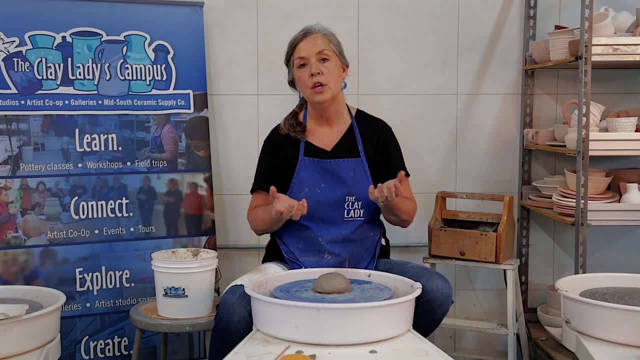 wheel and then they get to paint them with my clay paints, which are prepared slips. We let the project become bone dry, maybe clean the bottom a little bit, dip them in a clear glaze And just do that single firing so I can get the pots back to them in 7 to 10 days. 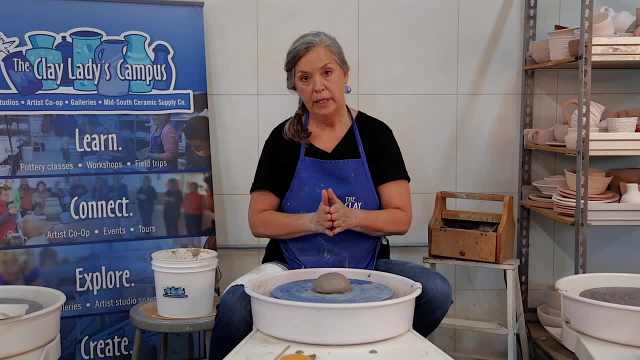 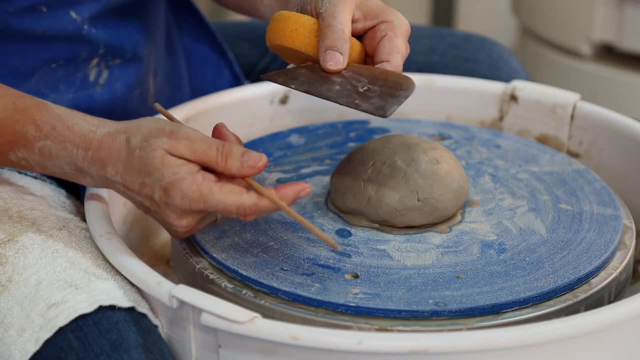 Now, when I get all the kids at the wheel, I explain to them the three tools that we use. That we have a sponge, a wooden rib and a shish kebab skewer. We call it a wooden tool, And then we put that in the water And then we talk about the clay, And then when 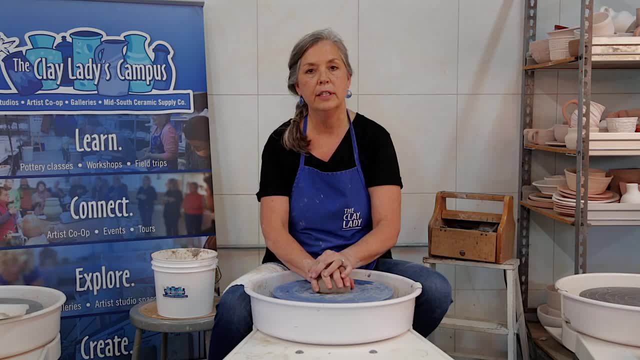 they're sitting at the wheel, it's really not the clay that they are controlling. That they're actually controlling invisible forces around the clay. That they're controlling friction by always keeping the clay in place, By always keeping their hands wet. That they're controlling centrifugal force by their wheel speed, The thinner the walls. 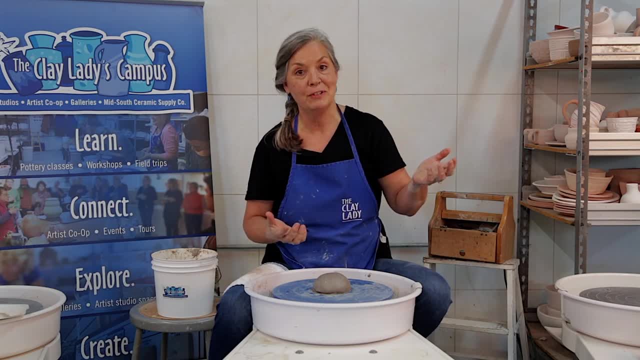 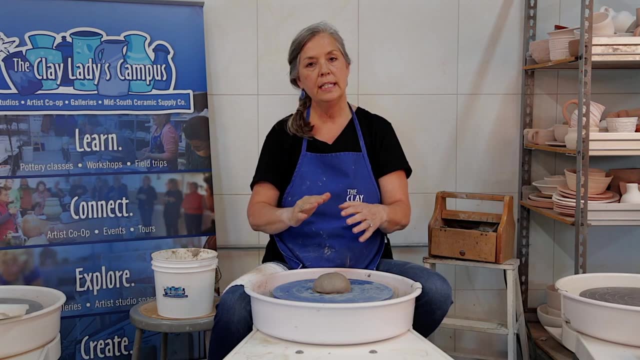 the slower the wheel, Or if they feel out of control, they probably are slowed down And we're also controlling gravity. The same thing that's holding me down in my seat right now is pushing on the clay, So they need to think about their form as, like the arches. 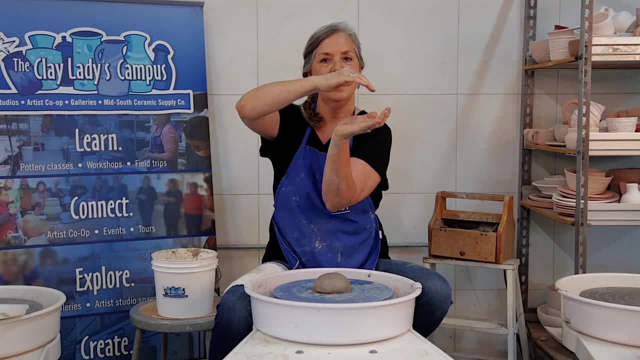 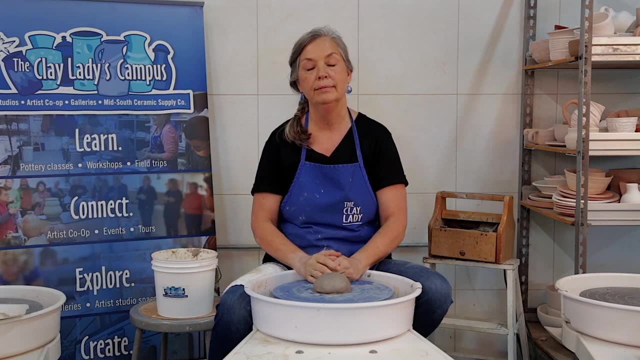 of a bridge, only that they're straight up and down, not side to side. Once we learn about those forces and that it really helps them know how to handle the wheel and handle the wall, Then I teach them the squirrel story. Now in my adult classes, we have nine weeks Each. 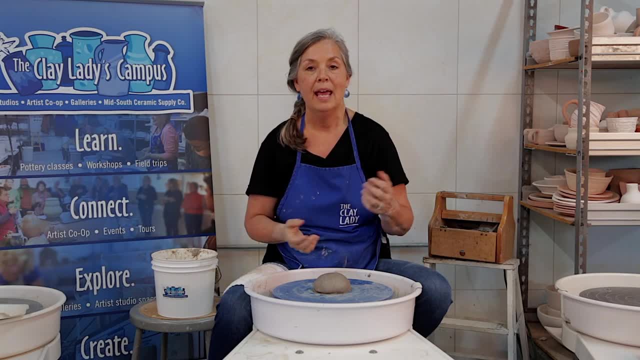 hand is doing something different at each of the nine steps, And usually it's the 8th or 9th week. Most of the adults have forgotten a step or two or a hand position or two, But I teach the kids how to be a squirrel. Perfect pottering position. They've got their. 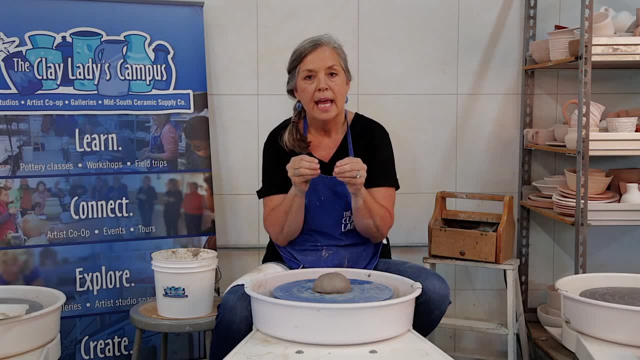 elbows tucked in, their wrists are loose, their hands are together And then we teach them that the clay is their acorn And then they're going to be the squirrel in the middle, And if he's got his teeth and his hands can't get together, they're going to program in. 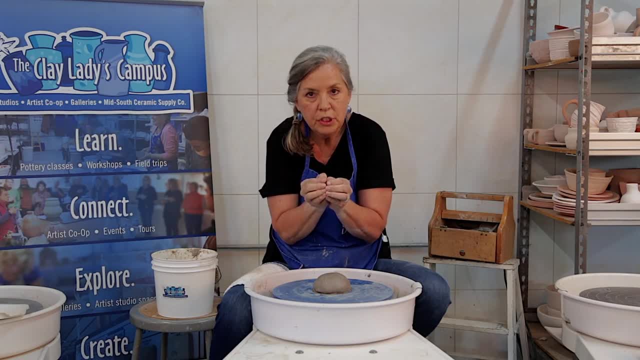 between. So that's how we handle the water and handle the water. Then I teach them the squirrel story. Now in my adult classes we have nine weeks. Each hand is doing something different at each of the nine and they're going to be a greedy squirrel which is centering. then they're going to crack open their 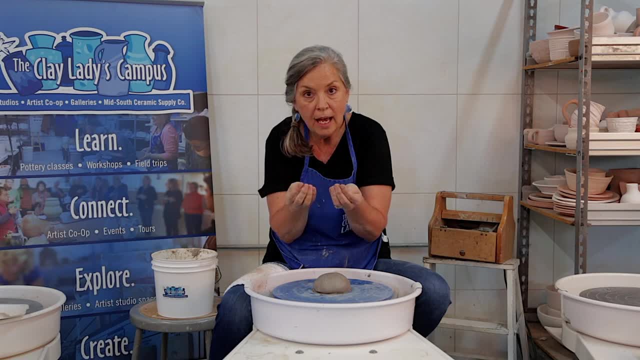 acorn opening. they're going to look inside, widening. then they're going to scoop out the shell, which is like an inverted pull. they're going to play with their food shaping. they're going to clean up after themselves because, although they're greedy and although that they 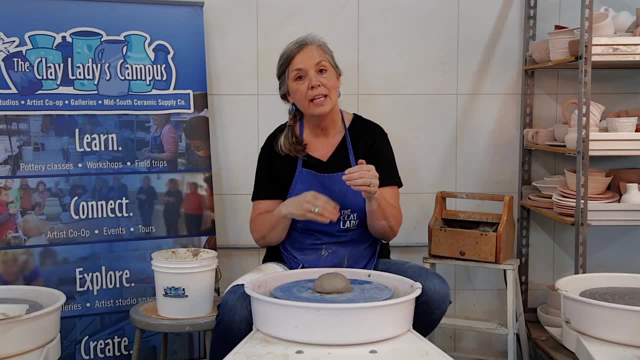 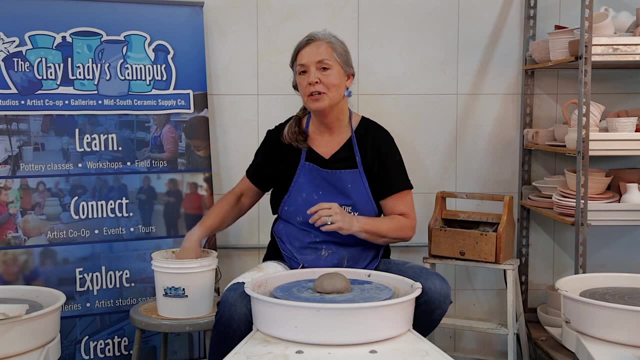 play with their food. they always clean up after themselves, and after they clean it up, they can paint it, of course. and then we pull it off the wheel and then the coach becomes the pop. so let me show you that squirrel story. so my hands are wet to control friction, my wheel speed. 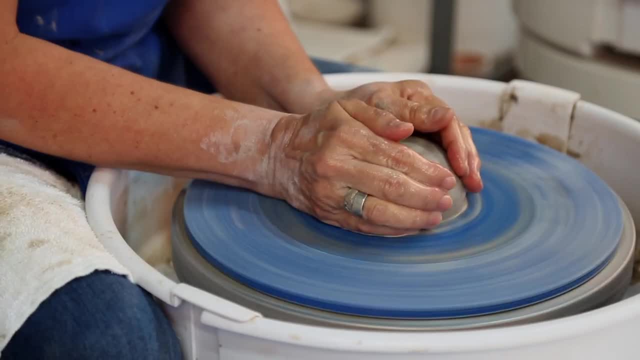 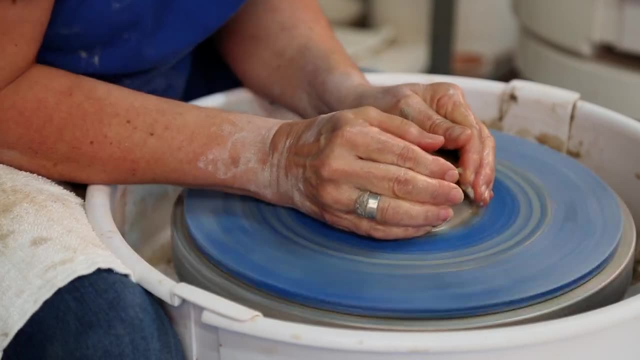 is fast to medium, because my clay is solid and i'm going to be a greedy squirrel. i'm going to push with the heels of my hands and the tips of my fingers and i'm going to push down with my thumbs. as soon as my hands get dry, i know that i need to get more water, and then i come back and 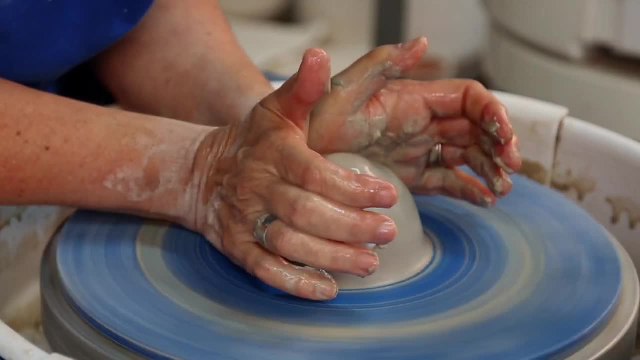 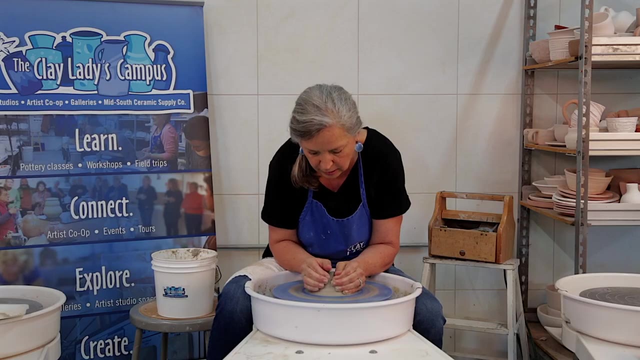 i'm a greedy squirrel. tuck those elbows in, push with the heel of the hands, pull with the fingertips and knees, thumbs flat down and squeeze. i'll have as young as five-year-olds standing next to the wheel, being greedy squirrels and being able to get their 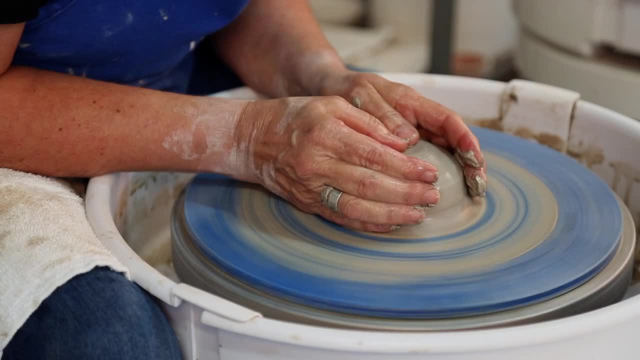 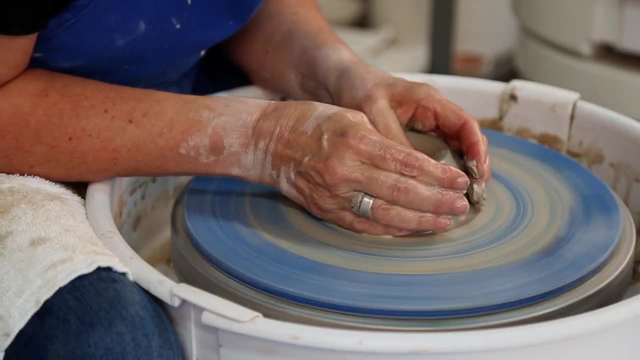 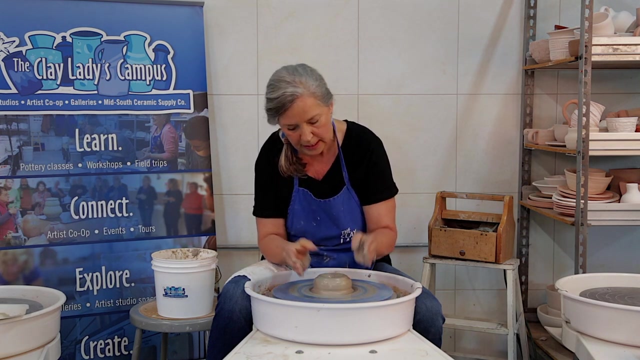 clay centered. once they get their clay centered, they use their thumbs to crack it open. as soon as they hit dry clay, they know to get water and they can go down. now i teach them to go to the top of their pinkies. that'll leave a good floor on your pot. so the top of their pinkies. that way, the top of their pinkies are going to leave a lot less floor. so they can't get the top of their pinkies, so they're going to get their top of their pinkies, so the top of their pinkies that. That way we know that the bottom is a good thickness. 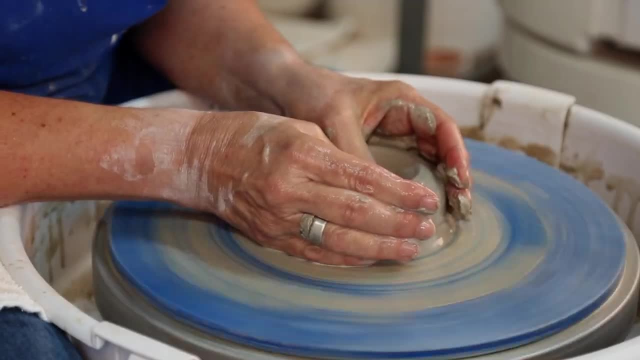 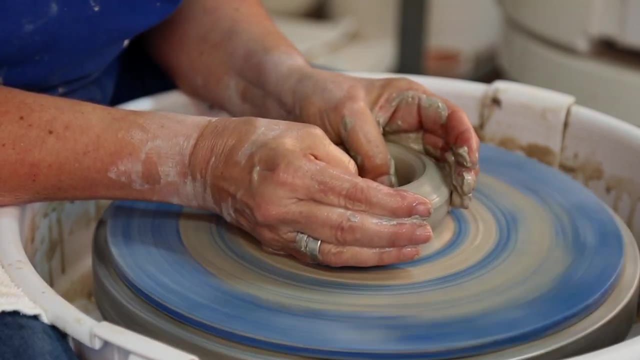 The walls are getting thinner, so I'm going to slow my wheel down, And after I crack it open, I want to look to see what's inside. So I'm going to keep my hands around my acorn and I'm going to slowly pull my thumbs into. 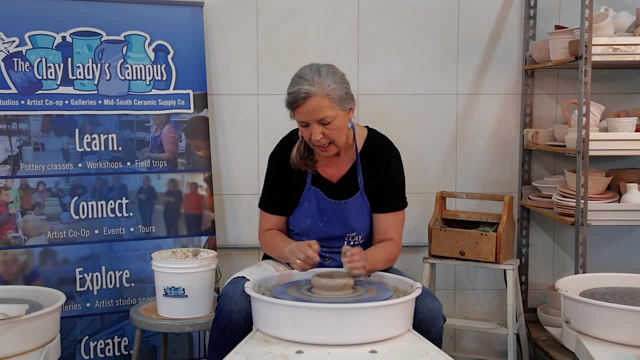 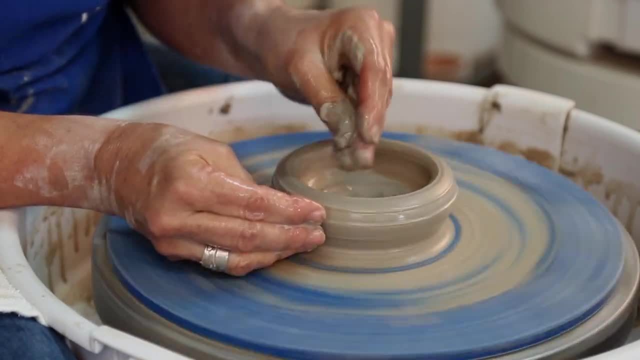 my hands. This creates a good defined bottom and a good wall for them to be able to pull or scoop out. When it's time for them to scoop out the shell, they need to make little squirrel hands. We're going to lean to the pedal because most kids don't know they're left and they're. 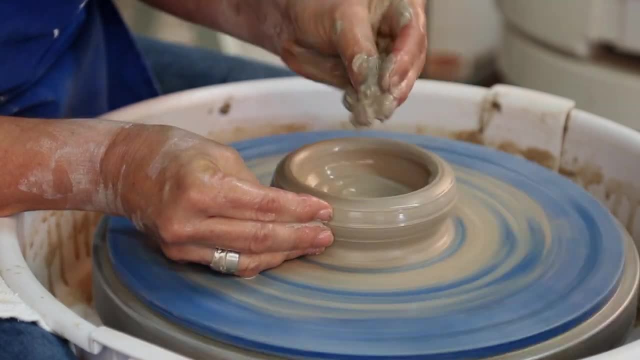 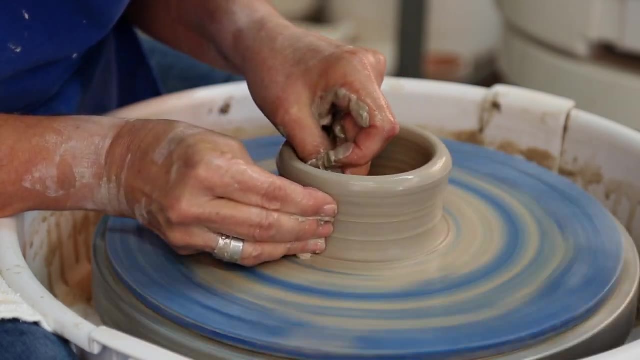 right And we're going to put one hand on the outside, the other hand on the inside, and we're going to go from the bottom to the top and scoop. The outside hand will follow the inside hand. This is a bit of an inverted pull. actually, it works really well because the inside hand 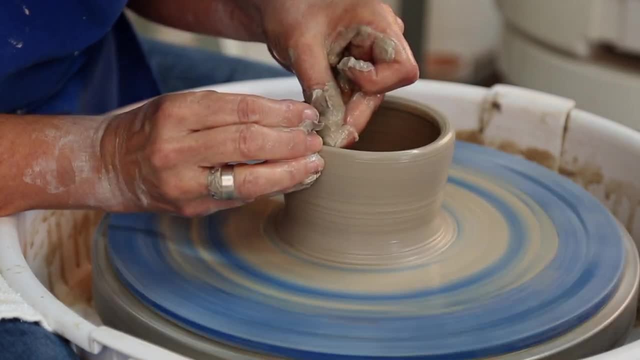 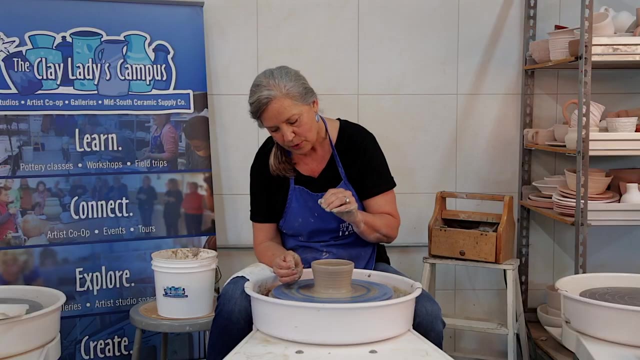 is being controlled by the outside hand, going from the bottom to the top. We want to scoop until the walls are thick as an Oreo cookie, Which is a clay lady rule, not a double stuff, not one you've already twisted in half. 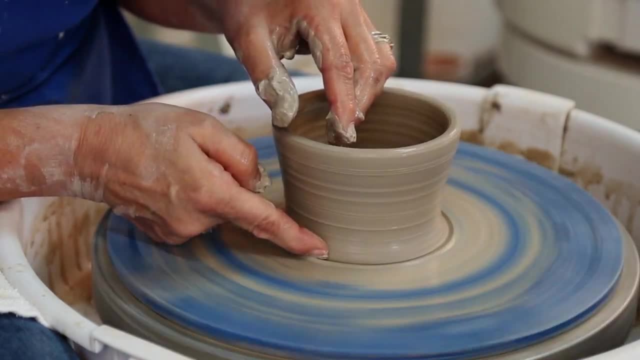 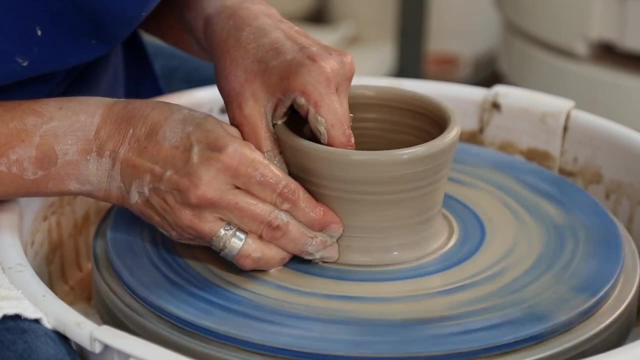 We want it to be just right Now down here. I call this the savings account, So we want to be able to get some of that clay up in our scoop. So we're going to make sure that our hands are slipping across the surface and we're 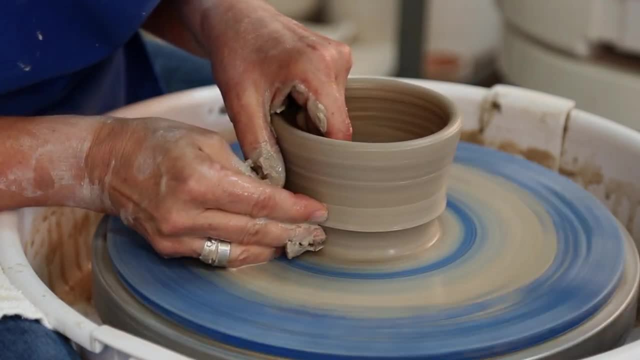 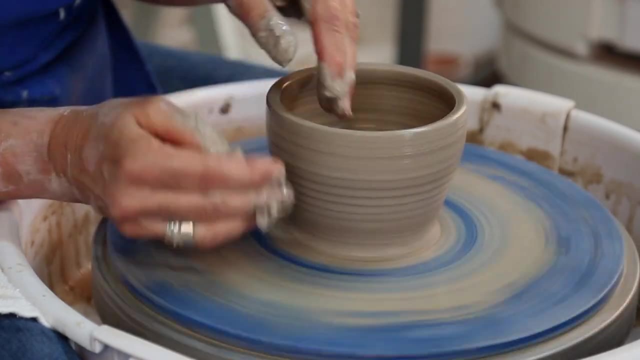 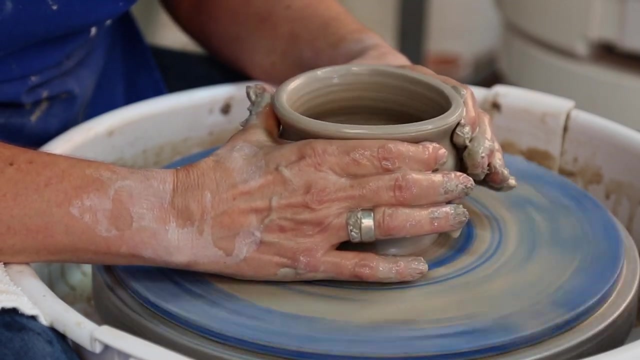 going to hold at the bottom and then do one more scoop. After they're able to scoop and get some height, then it's time to play with their food. And they can play with that shell by collaring, And we've learned that pots have body parts. 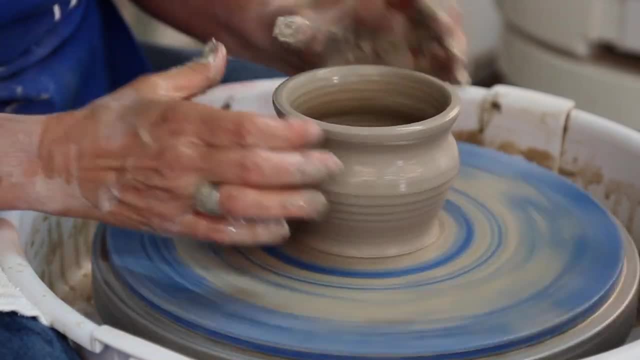 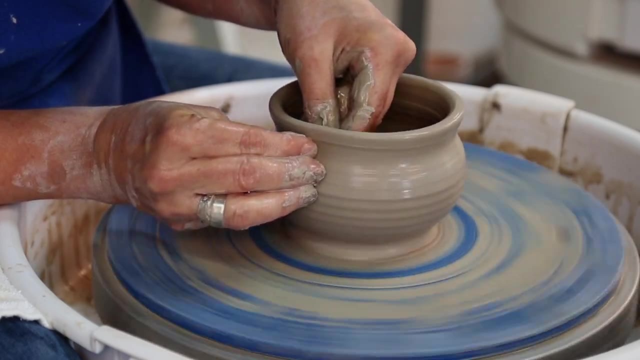 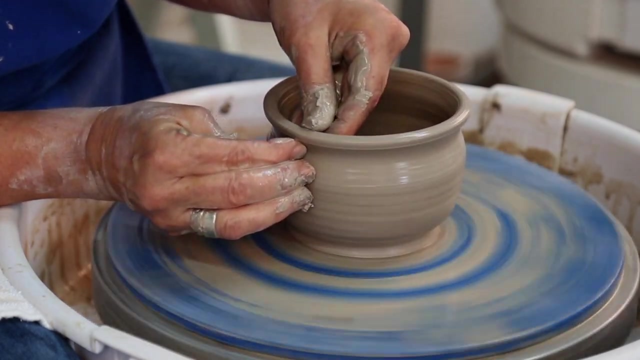 A foot, a belly, a shoulder, a neck and a mouth. Or they can make their little squirrel hands And if they want to make the belly bigger, they can scoop out and they can dance up the side of their pot. Once we get the shape that they want, it's time to clean up after ourselves. 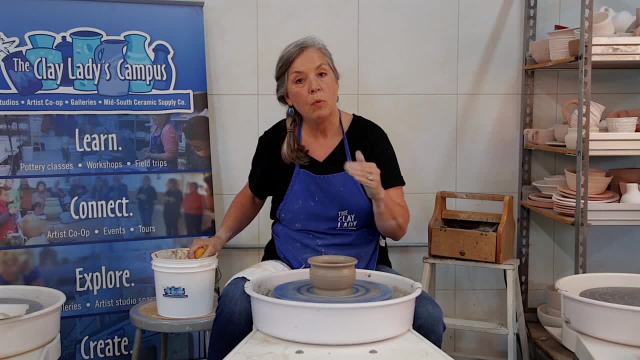 And so what we'll do to clean up. We want to make sure that there's no water in the bottom. We want to make sure that the bottom is nice and tidy on the outside so that I don't have a lot of work to do when it's time to do that single firing. 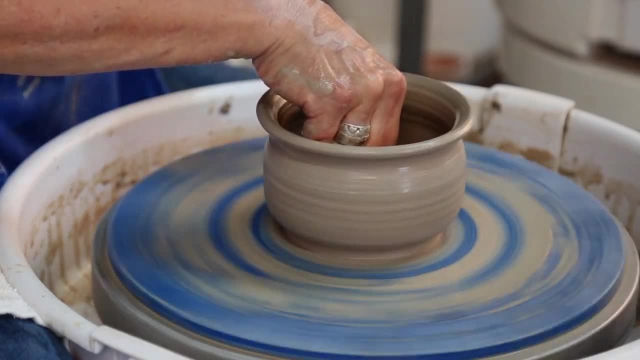 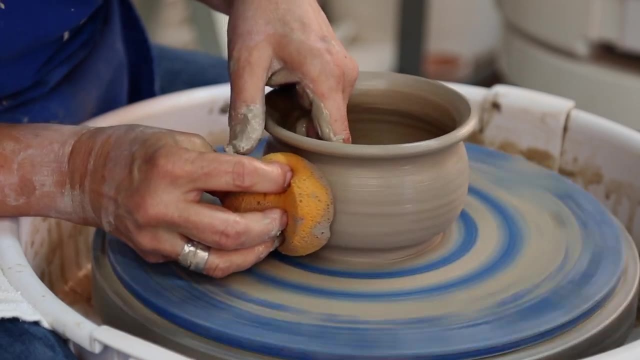 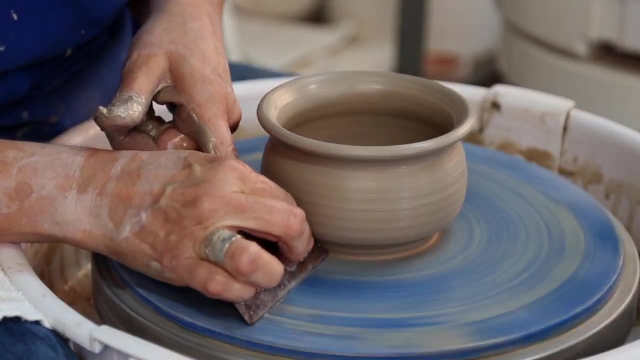 Also because the clay paints are actually prepared slips and they're watery. we want to make sure that the clay is dry so that when they paint on the wheel that they're able to really get a good coating of that clay paint on. This is when the rib comes in to really tidy that up at the bottom. 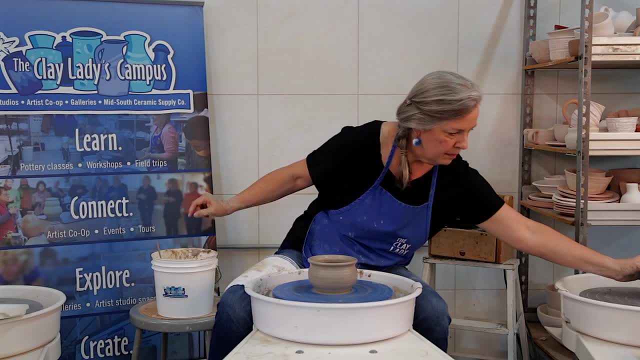 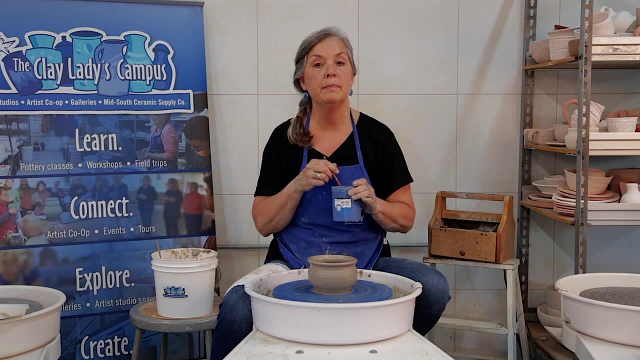 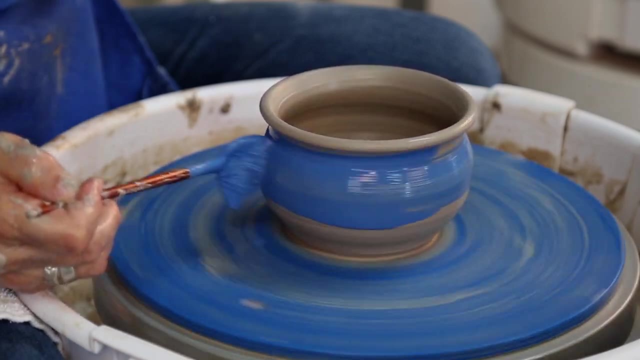 And then they can use my clay paints. My clay paints are just prepared slips. I have 20 colors for you to choose from. They're sold at Mid-South Ceramic Supply here on the campus. They really enable a teacher to have a good clay program because they're inexpensive.